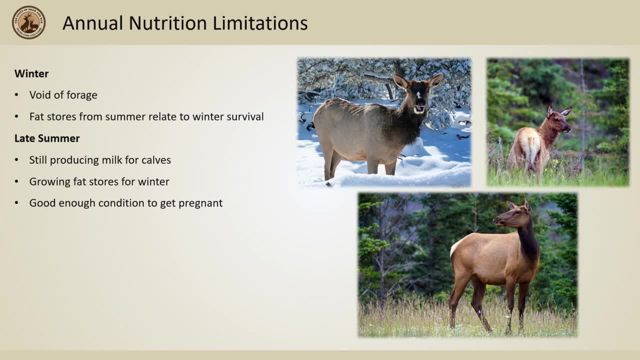 forage plays a vital role in elk survival. Late summer is a time when female elk are still producing milk for their calves, trying to put on enough fat to survive the upcoming winter and trying to be in good enough body condition to get pregnant and give birth in the spring. The 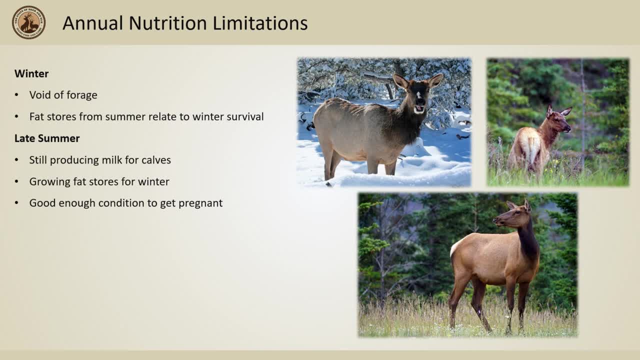 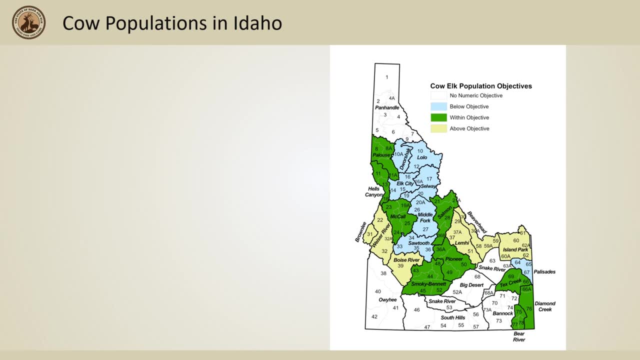 amount of fat that they have going into winter is closely related to their survival through winter and their ability to give birth in the spring. Cow populations across Idaho have fluctuated over the years. Currently, this is how the elk population has grown over the last few years. 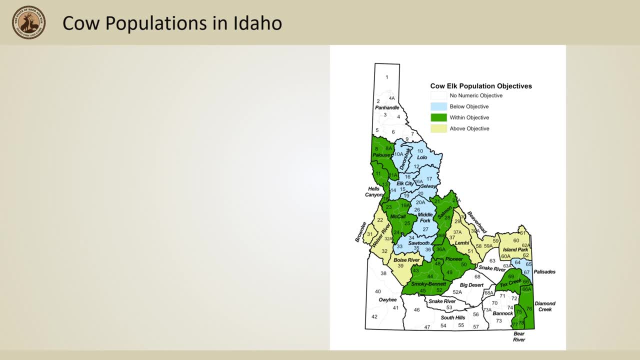 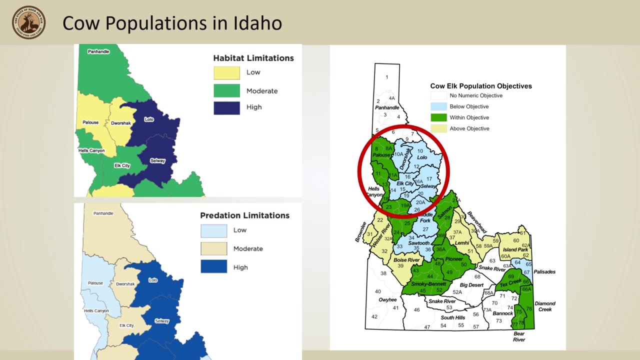 We will focus our talk on the northern portion, or the Clearwater region, where there are multiple zones below objectives. Reasons for these population declines can be a number of factors, such as harsh winters, drought years and many other stresses, all of which can play a role in. 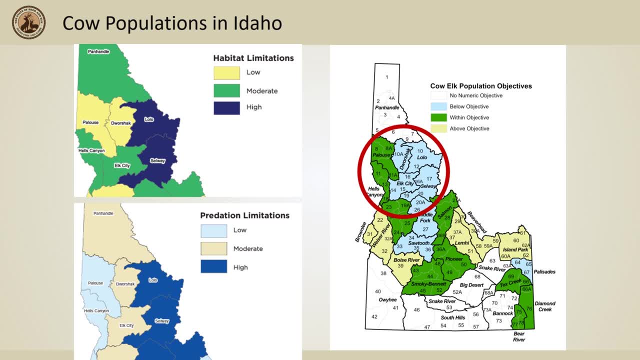 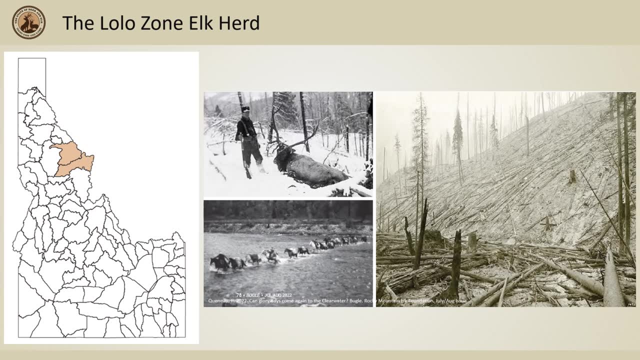 limiting the elk population, in addition to habitat or nutrition limitations. Within the Clearwater, the prized zone of the 70s to early 90s was the low-low zone. This herd boasted populations estimated to be as high as 16,000 animals in the 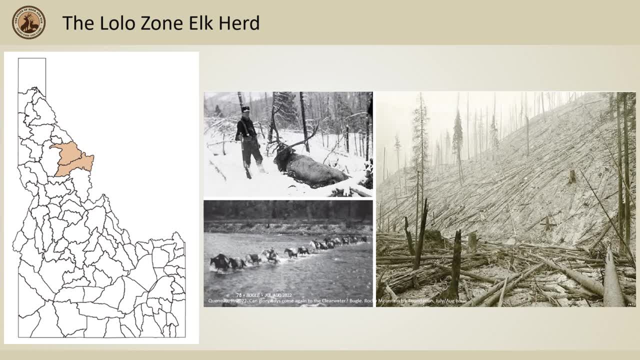 late 80s. Currently, the herd population is estimated to be less than 2,000 animals. These numbers were thought to be products of large shrub fields from the Big Burn era. During the mid-90s, many changes in both habitat and predators took place in this zone that could have led to this. 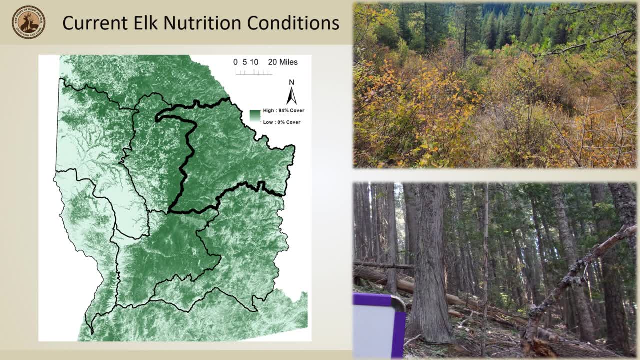 decline. Over the past four decades, the Clearwater region has lost the majority of population. Stands that used to be brush fields are full of shrubs, wildflowers and grasses are now thick timber stands, with little light penetrating down the dense canopy. This 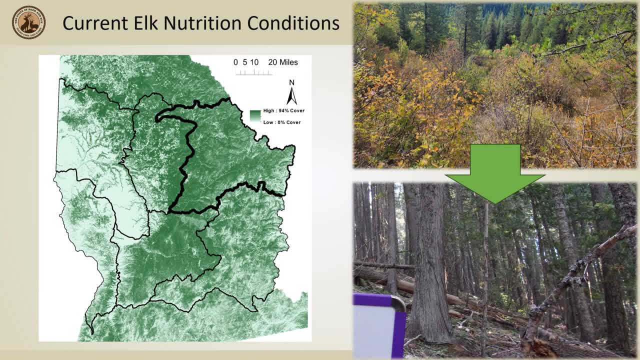 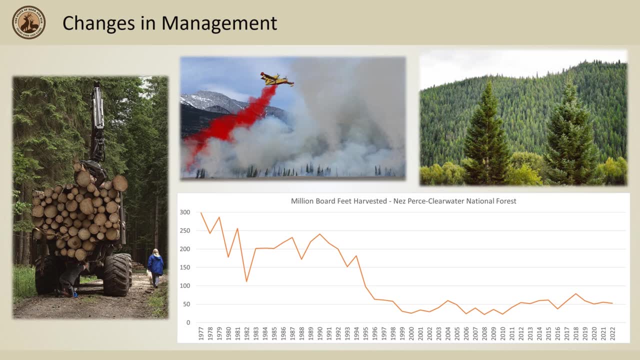 mid-to-old age forest bulge has left little areas for elk to find the required forage needed to sustain themselves and grow herd numbers. Reasons behind this loss of young forest stands could have been from our increasing ability to control and suppress fire. In addition, 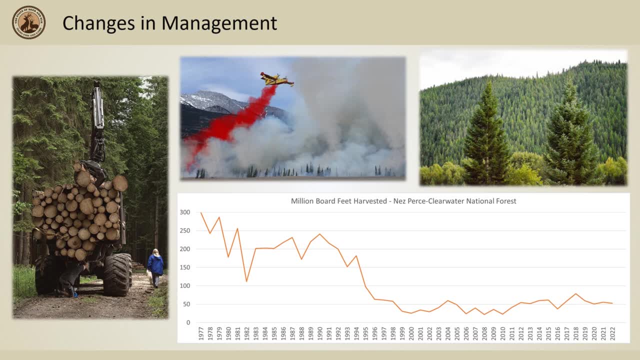 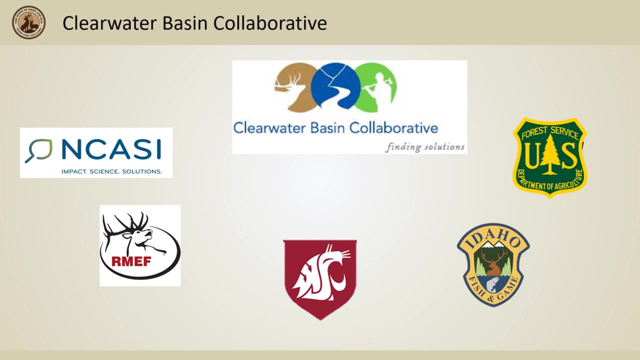 changes in timber sale management has led to a drastic decline in timber harvest on federal lands since the mid-1970s. Both of these factors could have led to the mid-to-old age forest bulge we are seeing today, To figure out why the low-low zone has continued to have population declines. 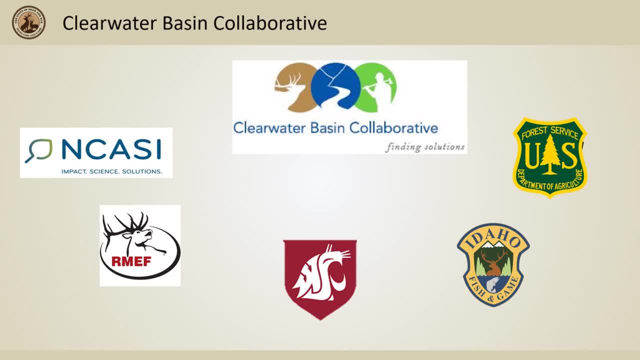 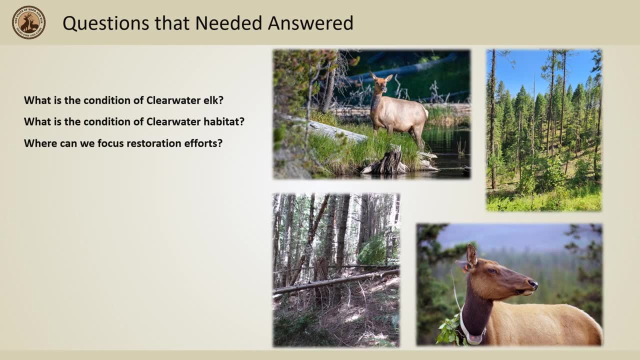 since the mid-90s and to understand how the current nutrition conditions across the Clearwater has affected elk. in 2013, the Clearwater Basin Collaborative was formed. Questions that they hoped to answer were: what is the condition of Clearwater elk? 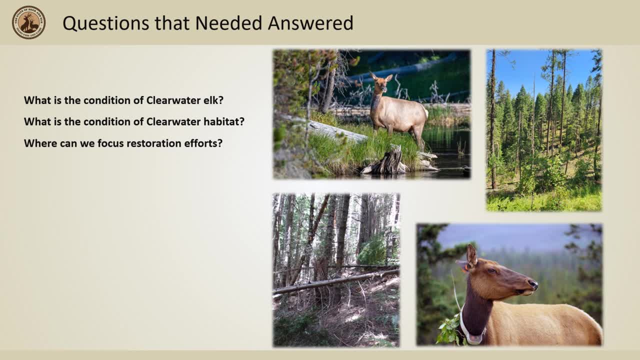 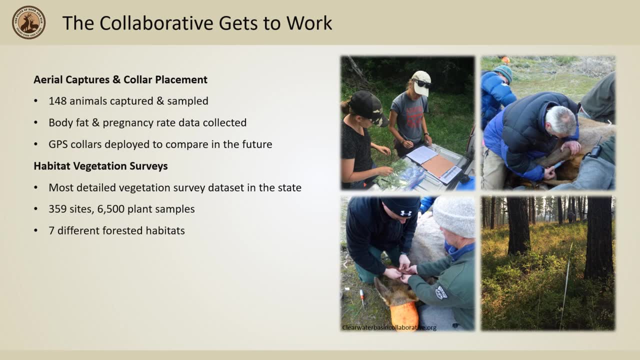 what is the condition of Clearwater habitat and where can we focus restoration efforts? To answer the questions posed to them, the Clearwater Basin Collaborative enacted the help from various elk nutrition experts. 148 cow elk were sampled for pregnancy rates and percent. 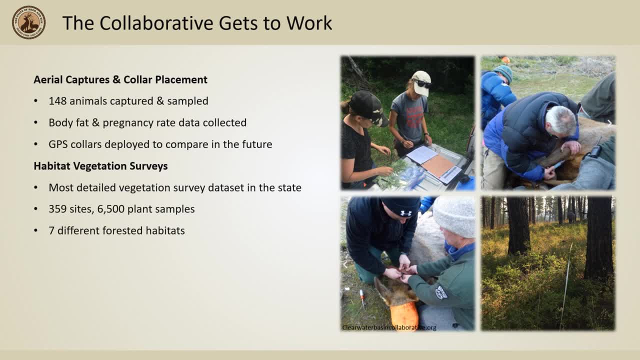 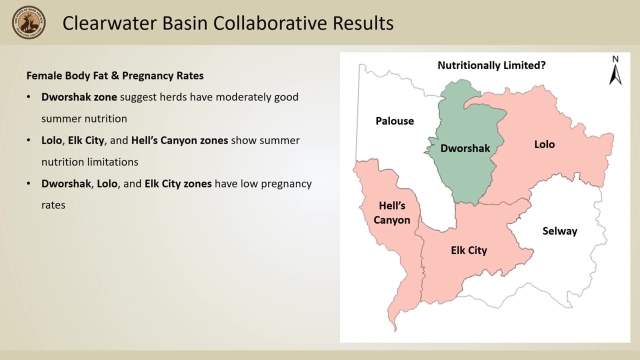 body fat across the herds in Clearwater. In addition, the Collaborative also conducted a multi-year vegetation survey. This vegetation data set is the most detailed collection effort in the state. Results from the Collaborative's efforts to measure body fat found that the Dorshak zone was the only zone in the Clearwater that had moderate 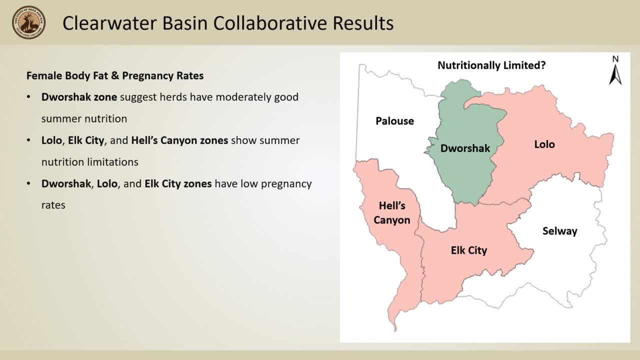 good summer nutrition. The remaining zones- low-low, Hell's Canyon and Elk City- showed low body fat percentages linked with summer nutrition limitations. When looking at pregnancy rates, Dorshak, low-low and elk city zones were seen to have low pregnancy rates. Low-low and elk city. 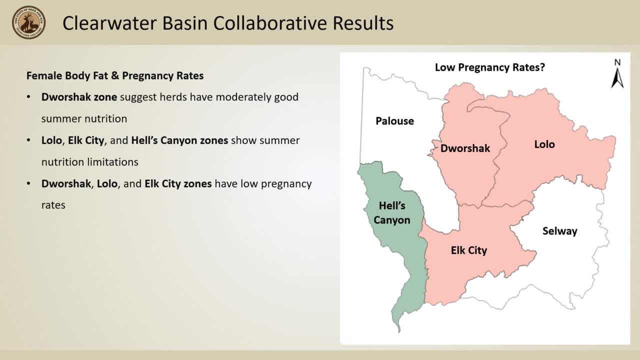 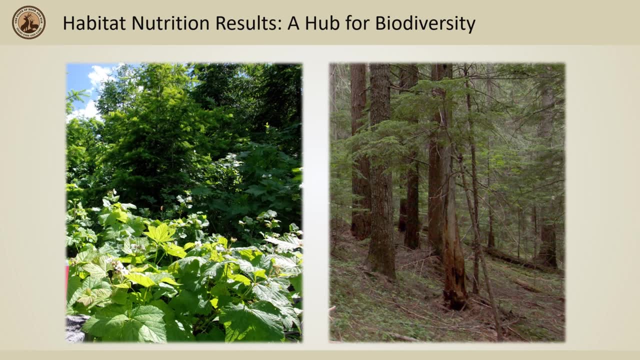 zones are consistent with what is to be expected with nutritionally limited areas. After completion of the vegetation surveys, key findings were determined. The Collaborative found that habitats such as Grand Fir, Western Red Cedar and Western Hemlock dominated forests that were less than 20 years old produced forage for elk that can be up to three times the amount. 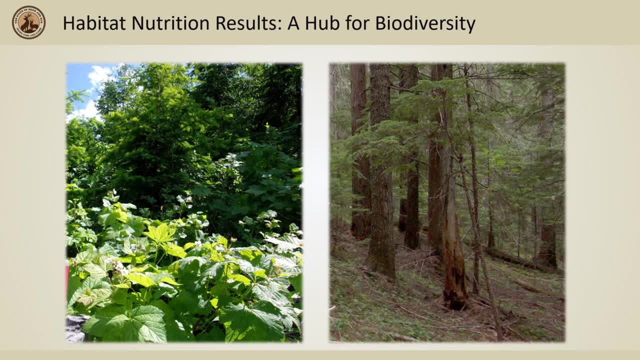 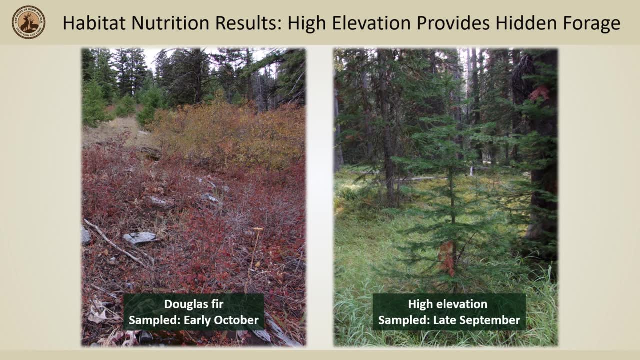 of forage produced in the same forest community over 20 years old. In addition, high elevation forests that are in wet pockets on north-facing slopes were found to retain healthier plants longer into the fall than in drier lower elevation forests. This example shows a Douglas fir forest. 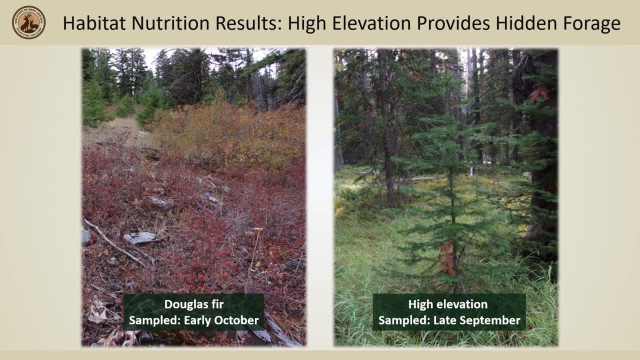 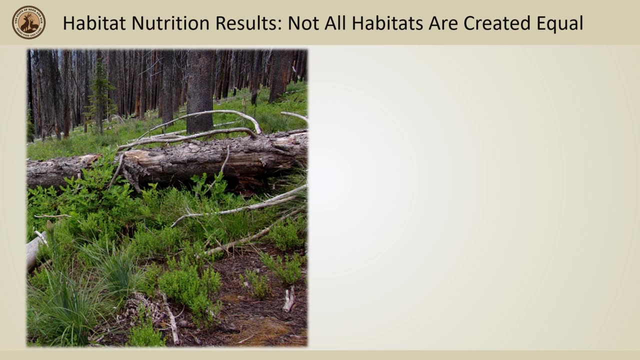 sampled in early October that is already lost its leaves to fall, versus a high elevation wet forest that was still green and luscious in late September. In all habitats there are plants that elk will strictly avoid eating. Some forests have more than others. This example is a high elevation. 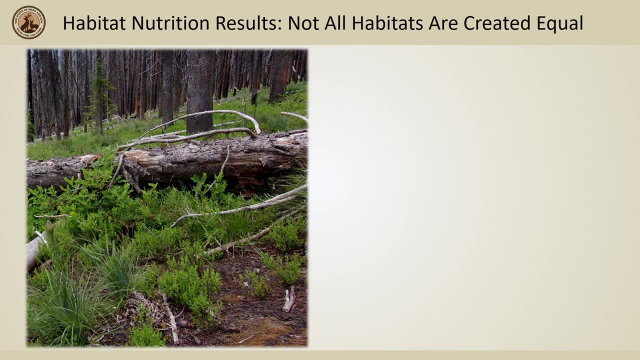 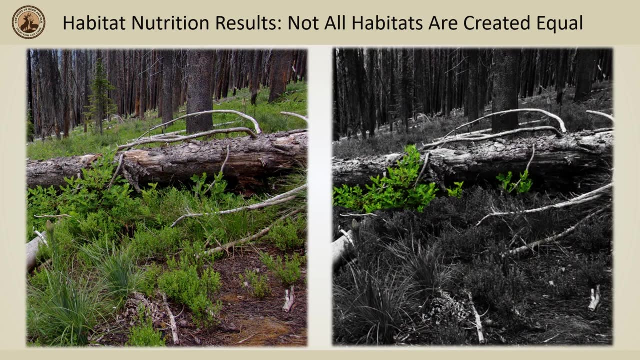 found on south facing slopes with dry climates, it appears there's great amounts of food available for elk. however, if you remove the plants, they don't eat and look at the same landscape from the viewpoint of an elk stomach, this is what is truly available for them: one single species. 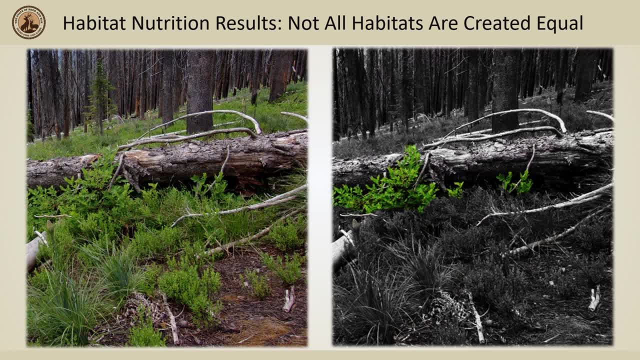 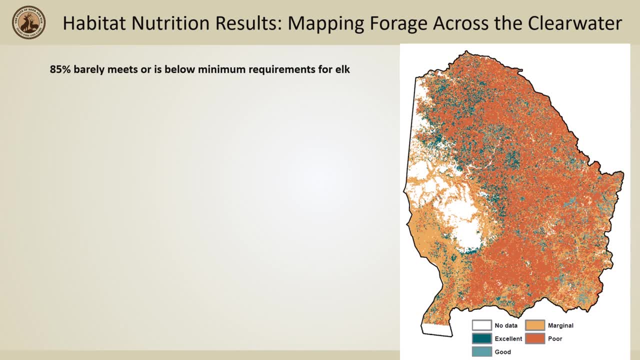 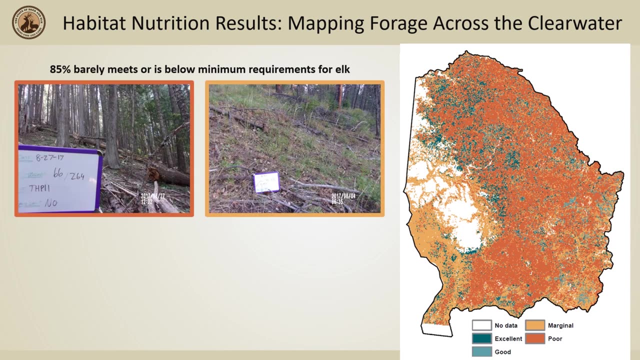 so even though it is green doesn't mean that elk will always eat it. in addition to understanding individual forested habitats, the clearwater basin collaborative was also able to create a map that calculates the amount of forage across the entire basin. in red and orange areas we have poor and 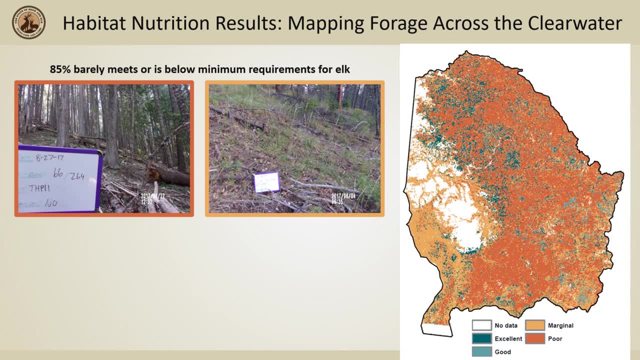 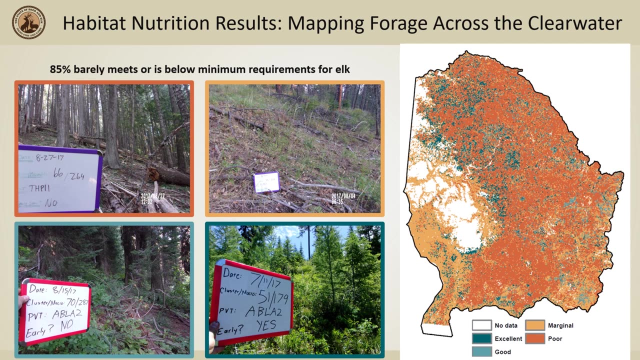 marginal nutrition. these areas just barely or do not even meet the minimum needs for a lactating female. in summer, these cows have nutritional limitations and have a hard time surviving winter and producing young. next are areas with good nutrition in teal and dark blue. they exceed the minimum requirements by a healthy margin, which provides cows with enough food to produce healthy. 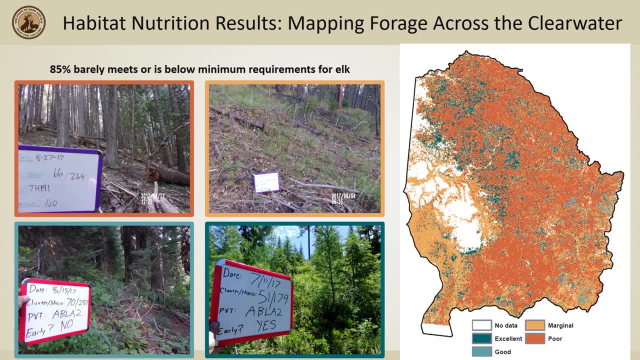 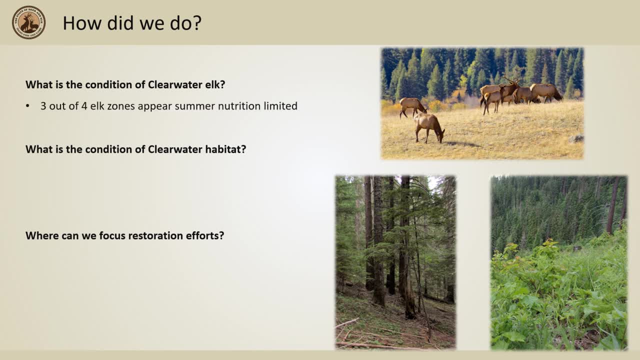 cows and produce enough food to feed their cows and produce enough food to feed their cows and produce enough food to feed their calves, survive with those calves through winter and have those calves survive to adulthood. the clearwater basin collaborative found the following answers: we now know that three out of four elk zones sampled appear summer nutrition. 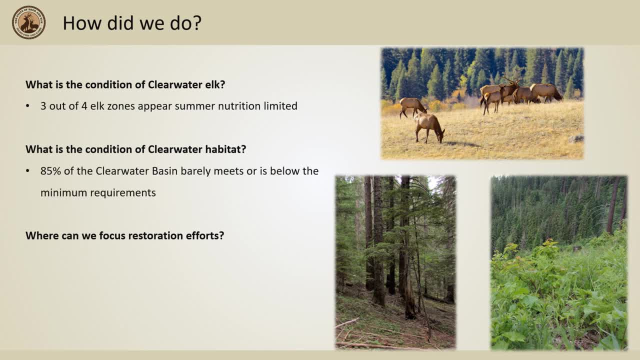 limited. at the end of the study, 85 percent of the clearwater basin barely meets or is below the minimum requirements for a female elk. and finally, by creating young forests in grand fir, western red cedar and western hemlock dominated forests, there is potential for large amounts of forage to be grown for elk. in addition, eastern elk zones such 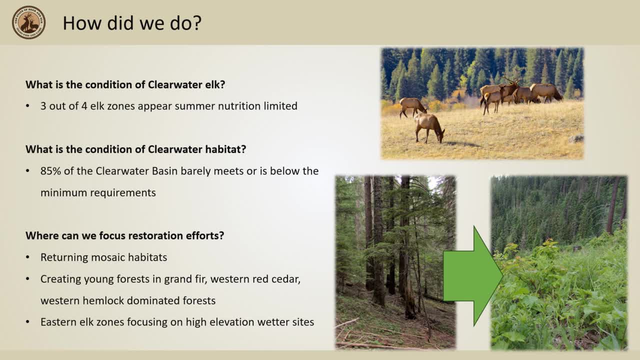 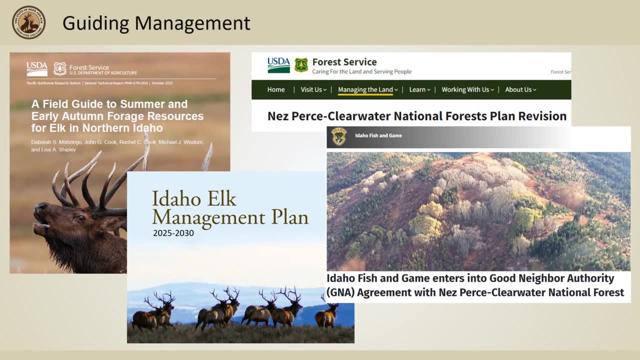 as the lolo zone could focus on high elevation wetter forests that provide more nutritious forage later into the summer than other forest communities. currently, this work has been integrated into various avenues to help guide land and population management, as well, as this information is being used to help guide project selection when working alongside the nez perce.